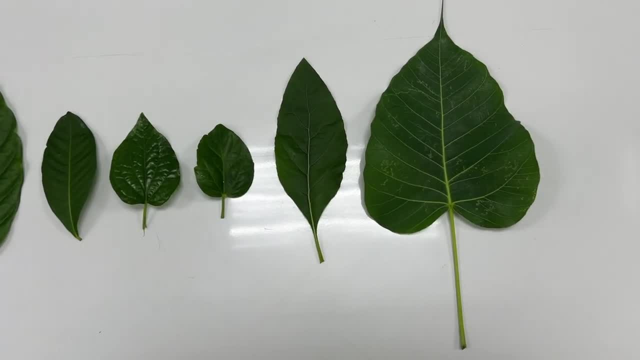 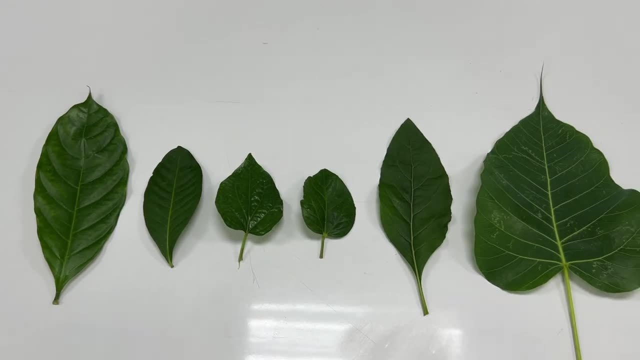 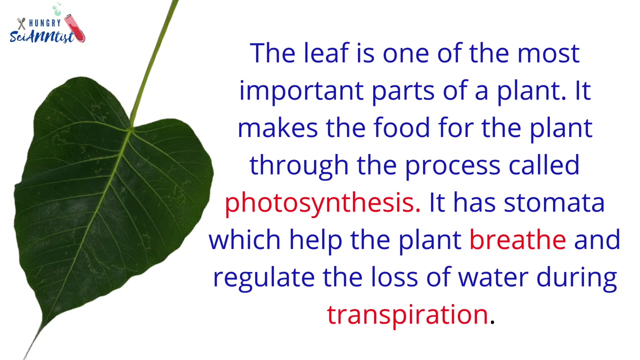 In this video we are going to learn the parts of a leaf and their functions. The leaf is one of the most important parts of a plant. It makes the food for the plant through the process called photosynthesis. It has a stomata which help the plant breathe. 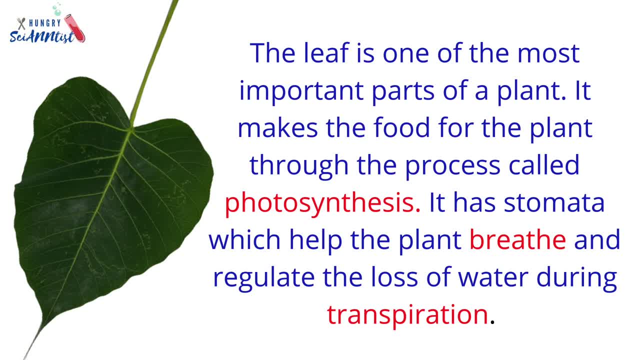 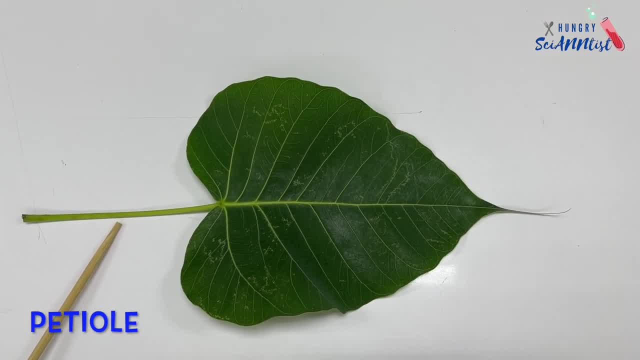 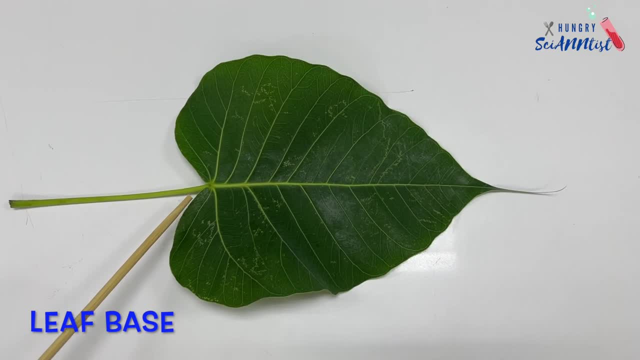 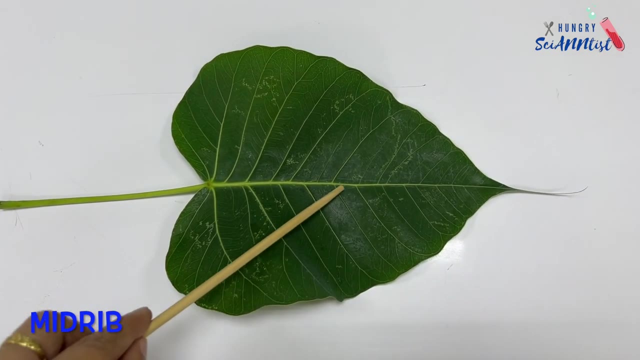 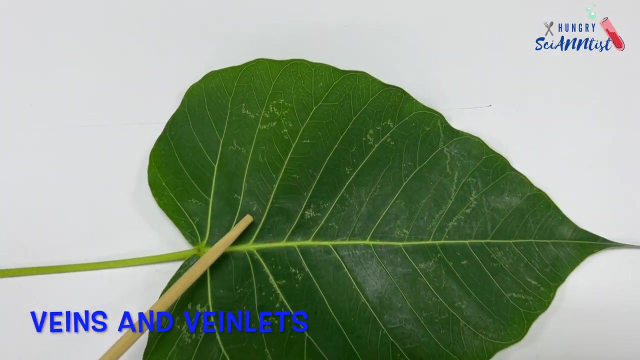 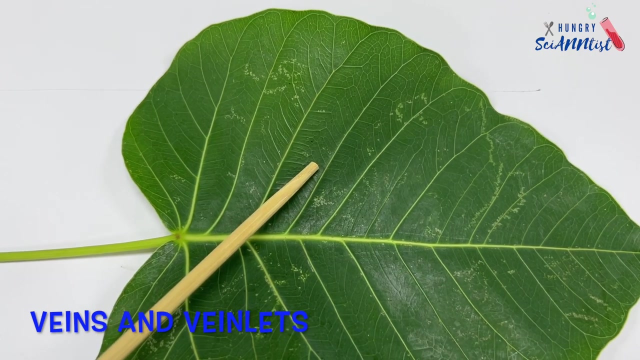 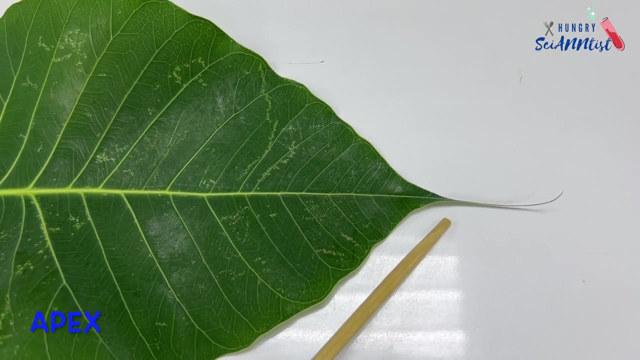 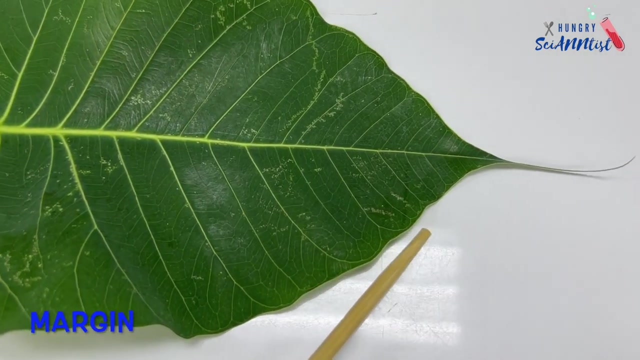 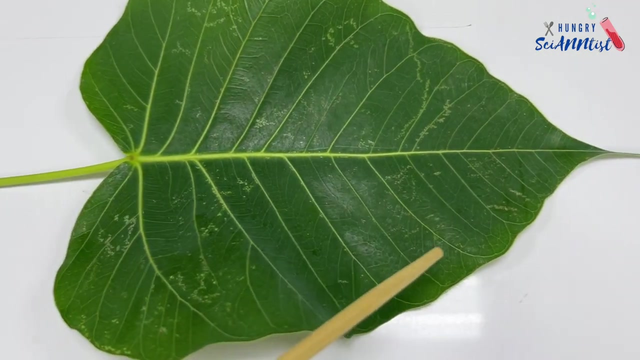 and regulate the loss of water during transpiration. This part is the petiole Leaf base. This part is the midrib. These are the veins and veinlets. This is the apex Margin And this whole part is what we call lamina. 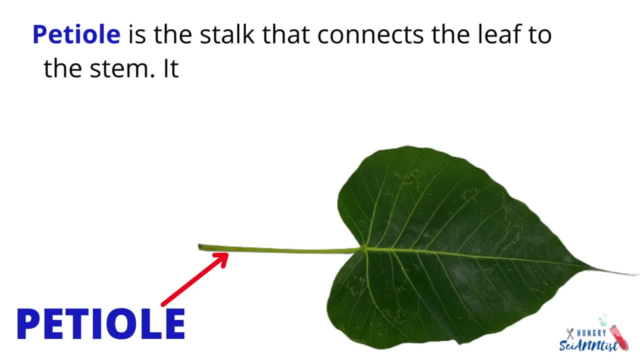 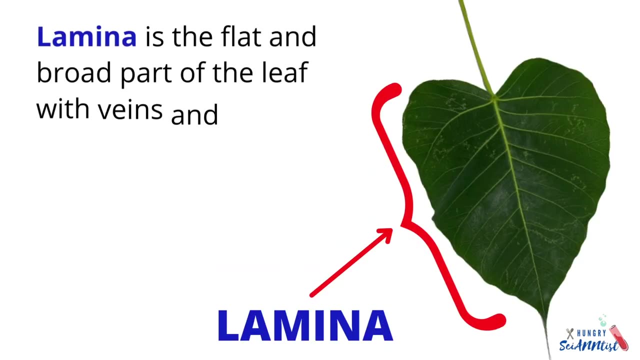 Petiole. Petiole is the stalk that connects the leaf to the stem. It is also known as leaf stalk. It holds the leaf to the stem and helps transport water and nutrients. Lamina Lamina is the flat and broad part of the leaf. 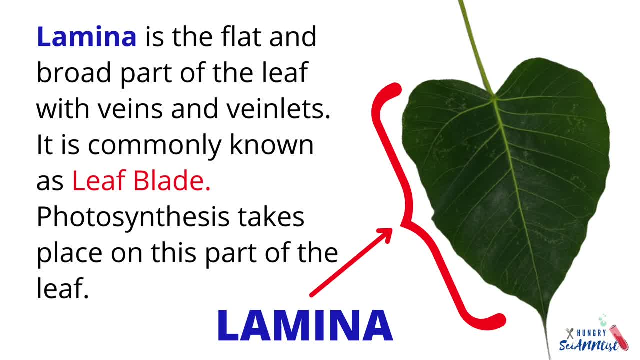 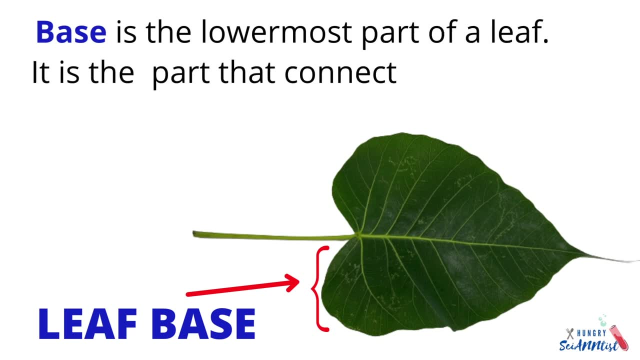 It is the leaf with veins and veinlets. It is known as leaf blade. Photosynthesis takes place on this part of the leaf: Leaf base. Base is the lowermost part of a leaf. It is the part that connects the blade to the petiole. 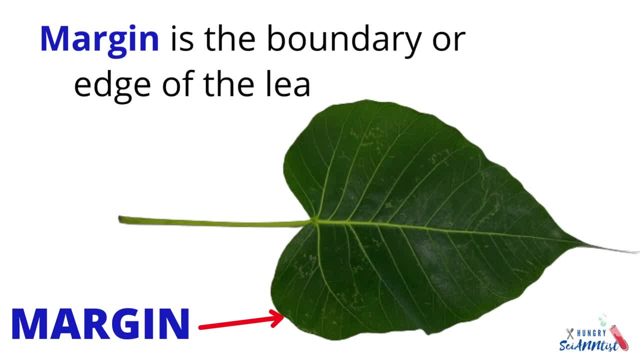 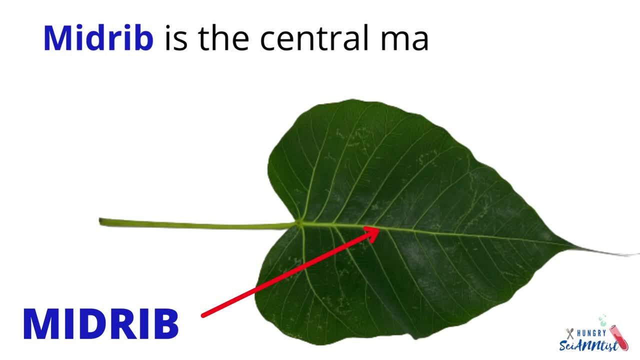 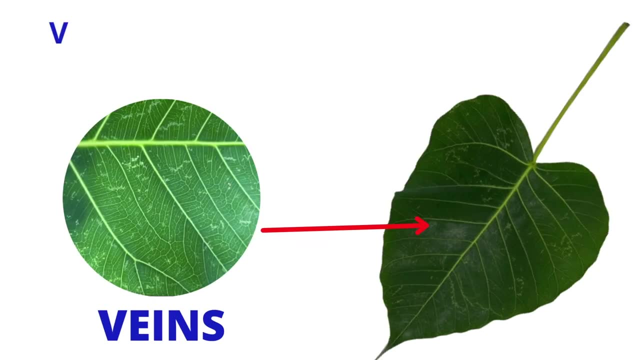 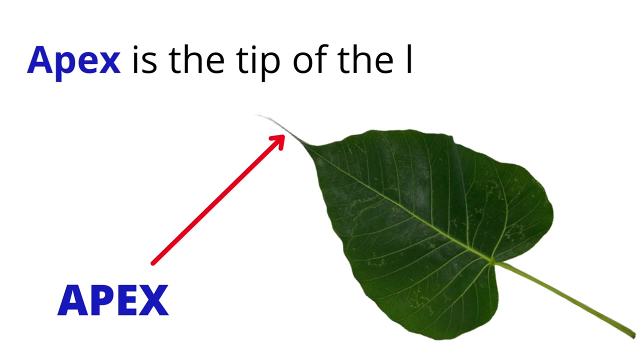 Margin- Margin is the boundary or the edge of the leaf blade. Midrib- Midrib is the central main vein that connects to the leaf stalk Veins- Veins are the vascular tissue bundles that support the leaf and transport nutrients. Apex- Apex is the tip of the leaf blade.